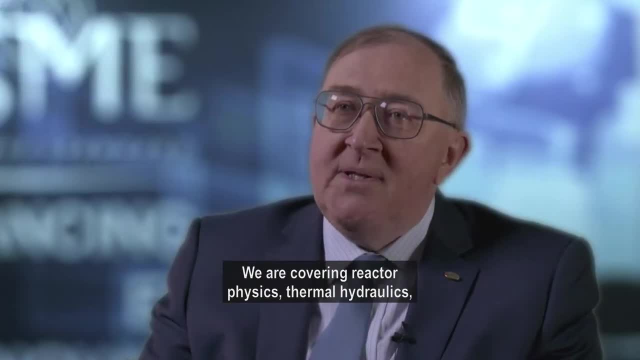 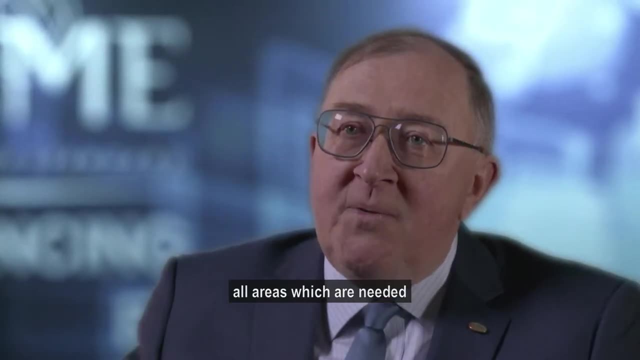 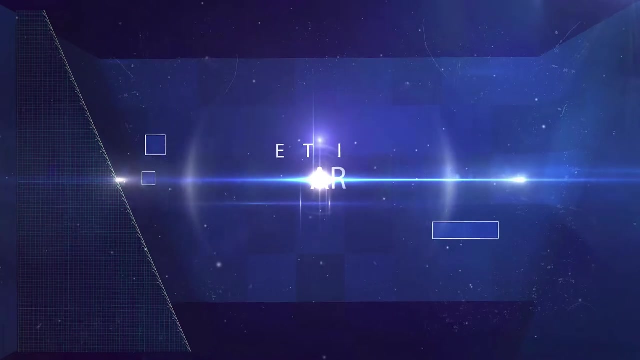 nuclear engineering and radiation science. We're covering reactor physics, thermal hydraulics, current plant operations, safety, nuclear education- all areas which we needed for nuclear engineering and radiation science to operate safe and to move forward with new reactor designs. How many associate editors are at theatu? 좋아amar naqadí 19902?. 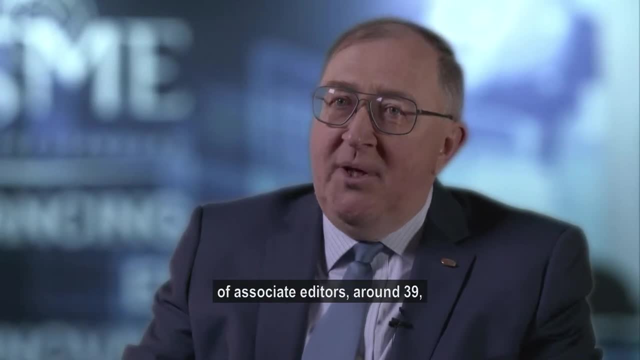 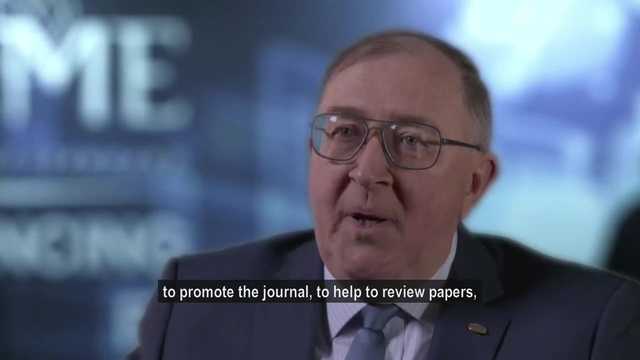 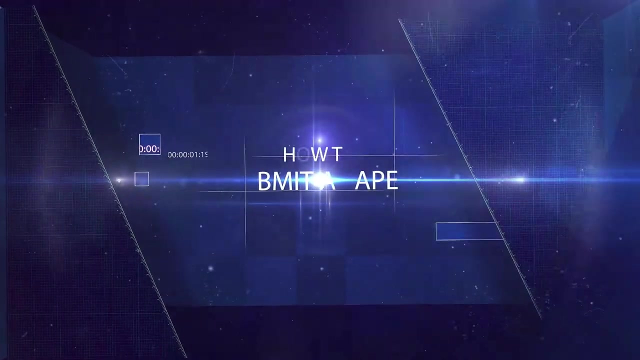 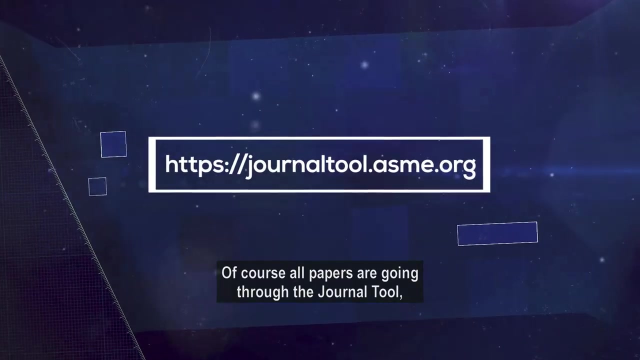 Captain Bogdan�� stretcher, with only two gäz hiçkeiten youtubers. How many associate editors are there? We have relatively large number of associate elevators- around 39- and 12 guest editors to promote journal, to help to review papers and to process papers through the journal tool. 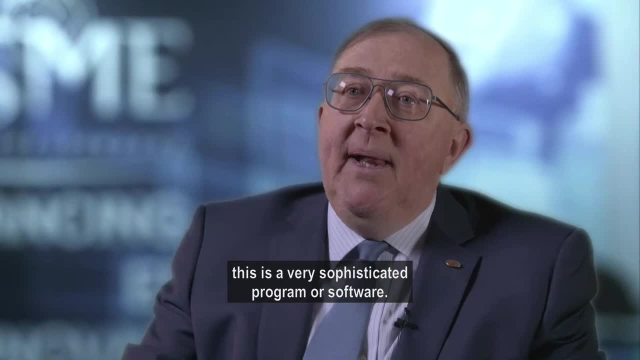 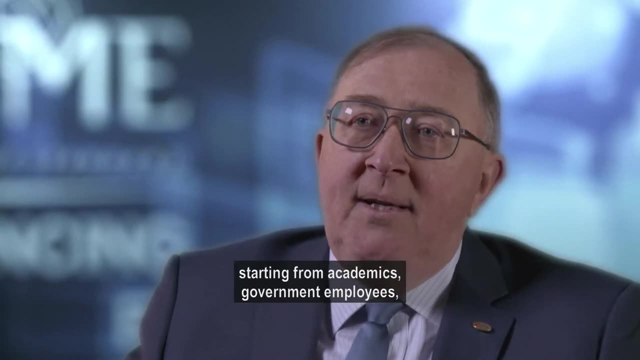 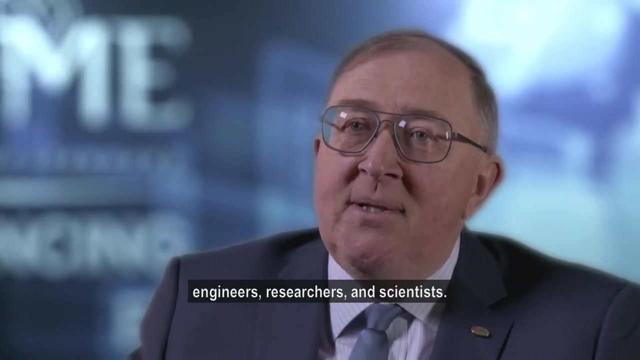 And also to attract new papers into our journal, very sophisticated program or software it helps author with through easy way to submit paper. we would like to hear from various areas, starting from academics, government employees with their ideas and everything, of course, experts in nuclear fields, engineers, researchers, scientists- also be encouraging students. 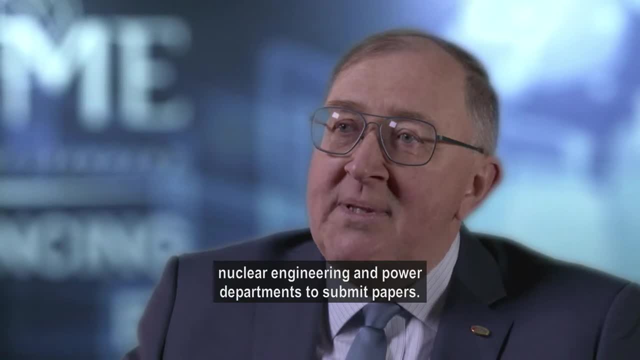 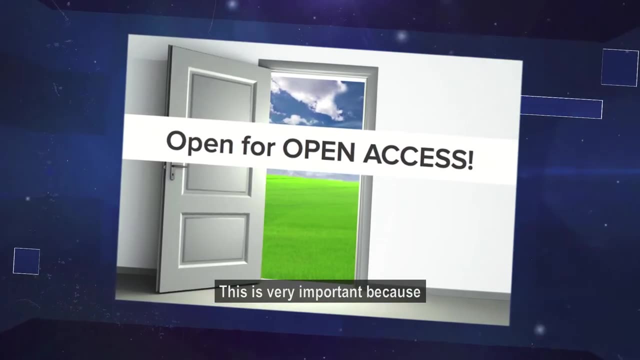 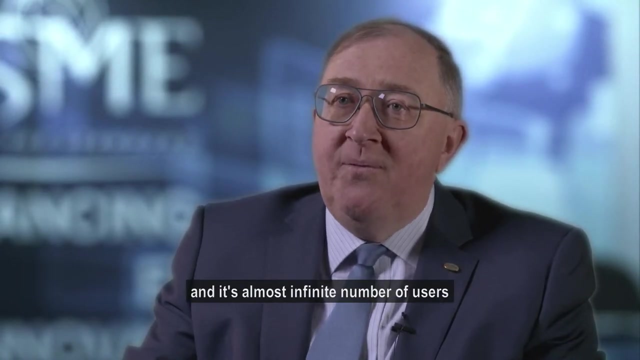 from nuclear engineering and power departments to submit papers. currently, we have option as open access for any of our papers. this is very important because it's helped to spread knowledge, the latest research around the world and it's almost infinite number of users and readers can be for these papers. I would 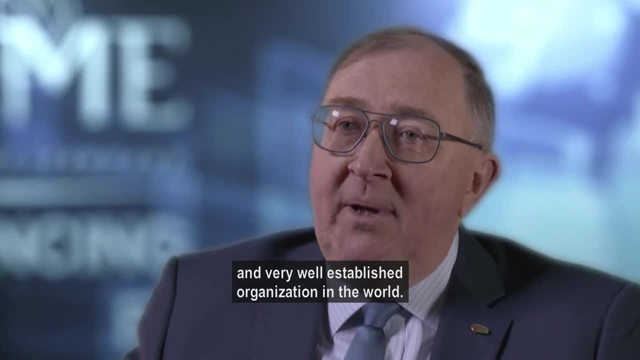 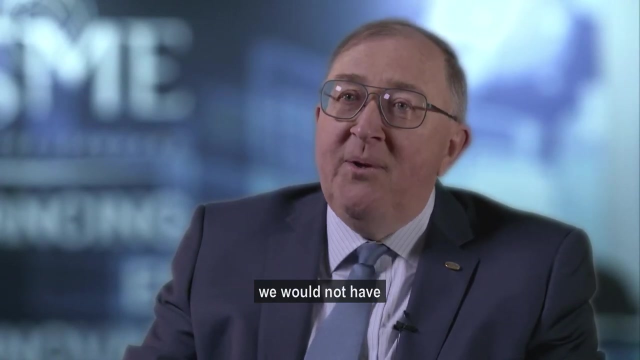 like to mention that SME is very well known and very well established organization in the world. codes and standards of SME using in many countries, which is very important. we have also some papers from developing countries, which is very important because without them we will not have a full, complete picture what we have in the world and many of them. 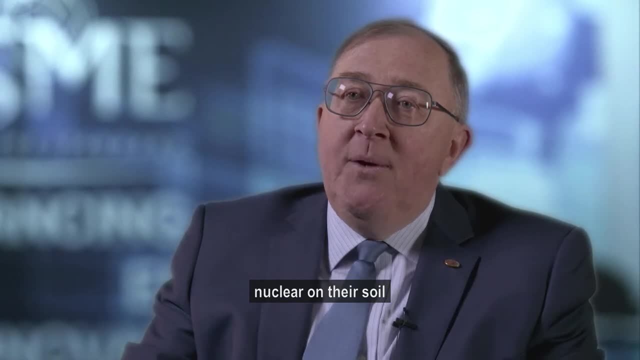 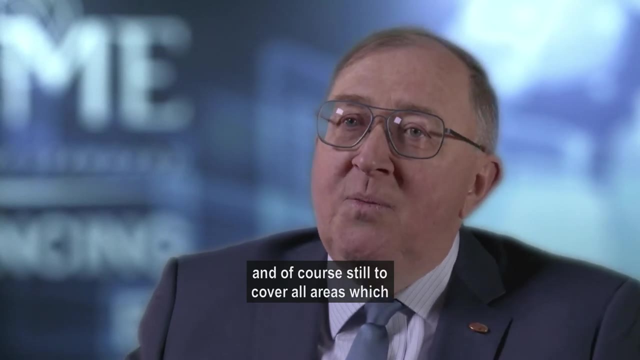 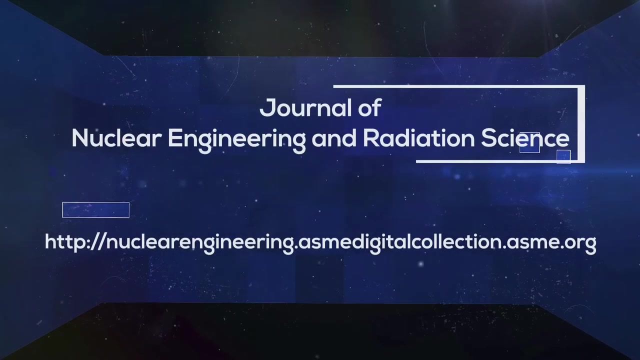 currently looking to establish nuclear on their soil. it is they working in these areas? this is what our vision and, of course, still to cover all areas which is will be new, for example, or appear, and within the nuclear engineering, radiation science areas. you.